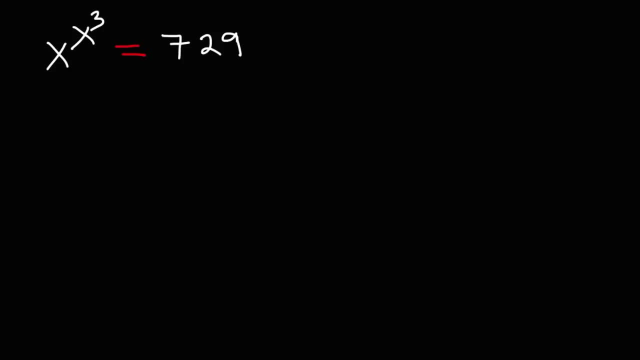 Consider this math problem: x raised to the x-cube is equal to 729.. What is the value of x? Now take a minute to try this problem, see if you can figure it out. And, by the way, for those of you, 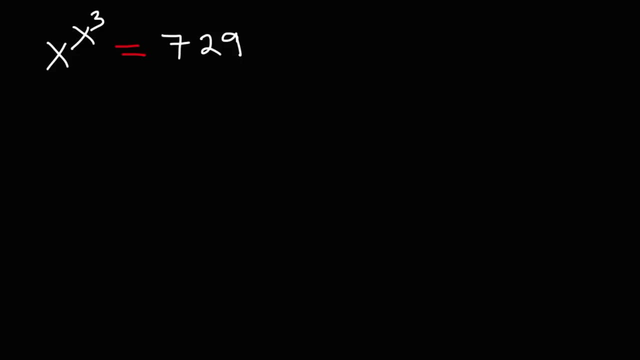 who want more challenging math problems like this one and others, check out the links in the description section below. I'm going to be posting more videos there as well. So let's get back to this problem. What is our first step? What do we need to do? What we want to do is we want to raise. 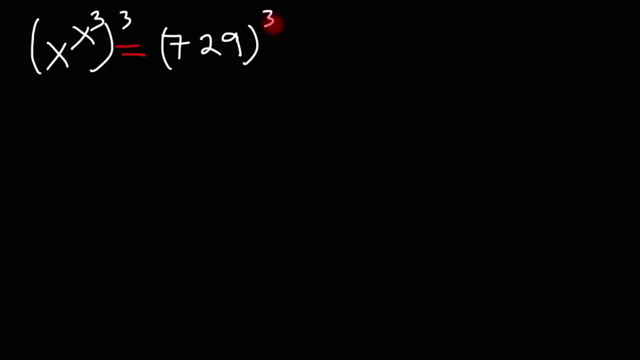 both sides to the third power. Now, if you're wondering why, I'll have to show you in a minute. Once you see it, then you'll know why. But for starters, it's due to the 3 that we see here, So we need to cube both sides of the equation. 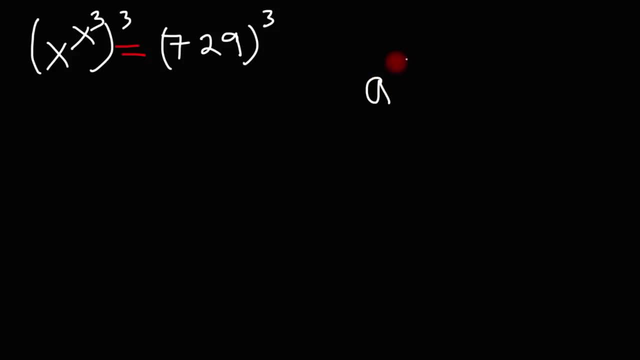 Now let's review exponents. For example, let's say: if we have a squared and we raise it to the third power, this is equal to a to the sixth power, because 2 times 3 is 6.. We can also reverse 2 and. 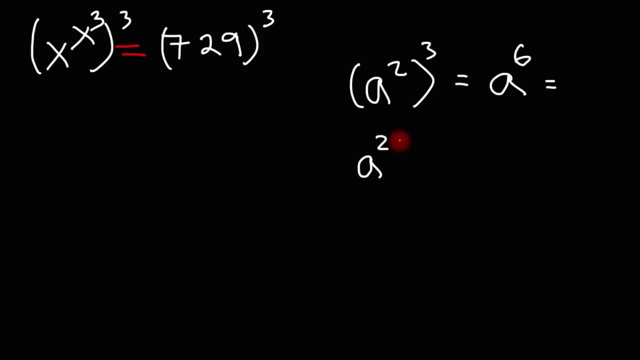 3.. So a to the sixth is a to the second times 3.. So we can also reverse 2 and 3.. So a to the sixth is a to the second times 3.. So we can also reverse 2 and 3.. So a to the sixth is a to the second times. 3.. So that's cubism, and it doesn't matter how big it is, because all of these coupledантs are the same thing. So if we assume, talking about the Karen equation, we can say that x is squared by x, squared raised to the third power. You can also break it down by x to the third times 3,. 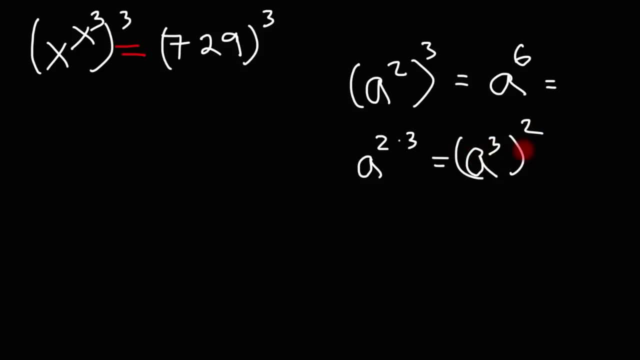 which we can write it as a to the third raised to the second power. So let's focus on what we have here. We have x cubed raised to the third power, or rather x raised to the x cubed raised to the third power. 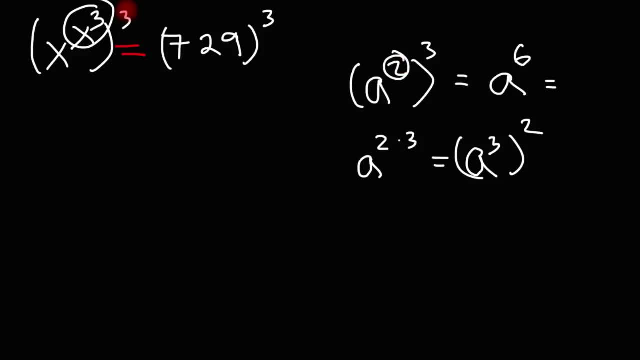 So this x cubed is like the 2, and this 3 here is like that 3, times 3, or x cubed times 3, or 3x cubed. So this expression on the left is equivalent to x raised to the 3 times x cubed. Just think about what we did here. 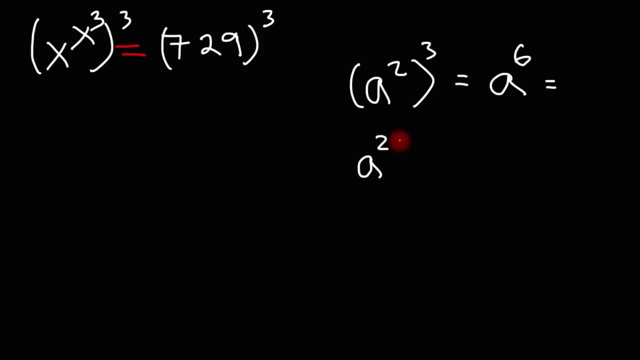 3.. So a to the sixth is a to the second times 3.. So we can also reverse 2 and 3.. So a to the sixth is a to the second times 3.. So we can also reverse 2 and 3.. So a to the sixth is a to the second times. 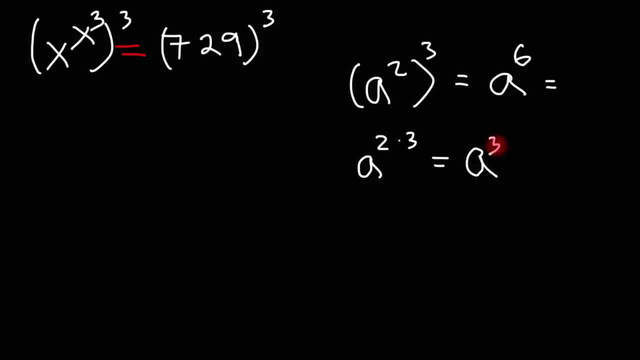 3. Which we can write it as a to the third raised to the second power. So let's focus on what we have here. We have x cubed raised to the third power, Or rather x raised to the x cubed raised to the. 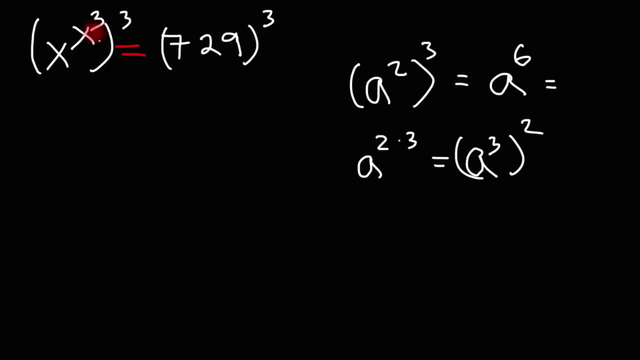 third power. So this x cubed is like the 2. And this 3 here is like that 3.. So I can write it as 2 times 3 or x cubed times 3 or 3x cubed. So this expression on the left is equivalent to x raised. 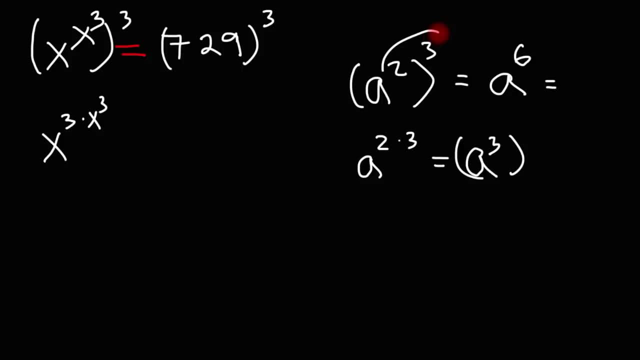 to the 3 times x cubed. Just think about what we did here. Now what I'm going to do is I'm going to rewrite this expression. So imagine taking the expression that we have here- 2 times 3, and write it as a to the third. 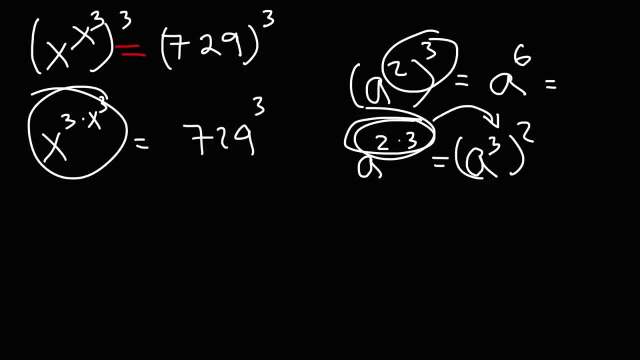 raised to the second power. So we can rewrite this expression as x to the third raised to the x cubed, Because when you raise 1x to the third, you're going to have x to the third, So you're going to have x to the third. 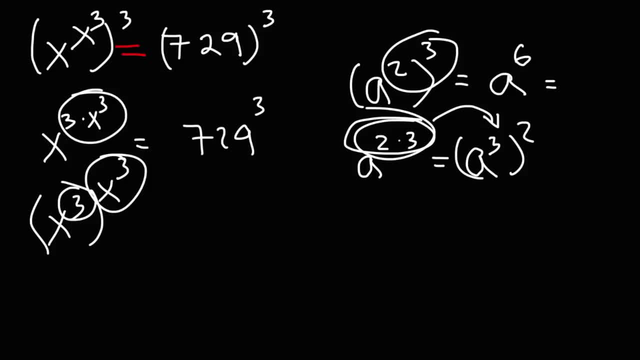 And when you're going to another you can multiply them. This is the same as 3 times x cubed. So what we did is we basically reverse the order of x, cubed and 3. Just like what we did here, We. 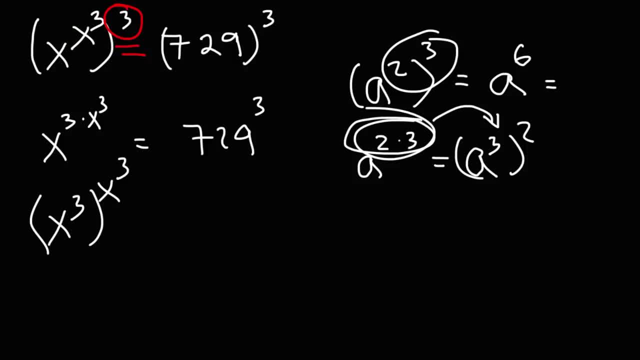 reversed the 2 and the 3. And we can do that. Mathematically both expressions are still equivalent, But notice that these two are in the same form. They're equal to each other: x cubed raised to the x cubed, And so what we want to do now is we want to multiply them And we want to 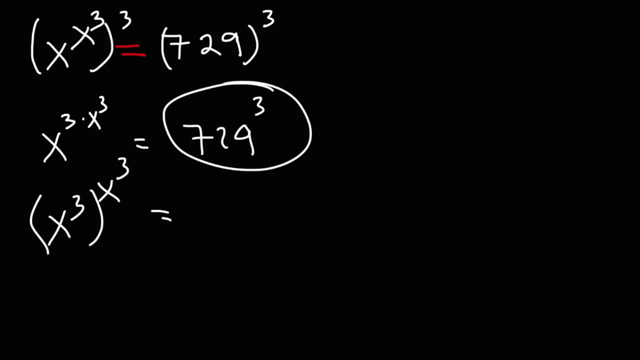 is change this expression such that we have a number raised to the same number. If we can do that, it's going to make this problem a lot easier to solve. Now, 729 is a cube of what number? 9 times 9 times 9 is 729. So it takes 3 nines to 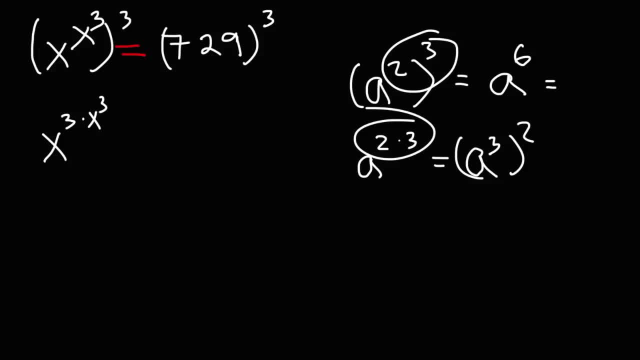 Now what I'm going to do is I'm going to rewrite this expression. So imagine taking the expression that we have here 2 times 3, and write it as a to the 3rd raised to the 2nd power. So we can rewrite this expression as x to the 3rd raised to the x cubed. 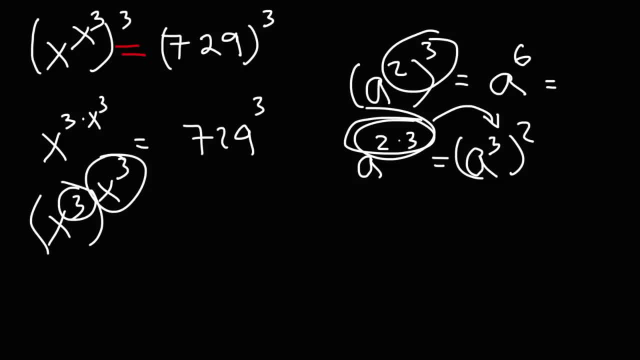 Because when you raise one exponent to another, you can multiply them. This is the same as 3 times x cubed. So what we did is we basically reversed the order of x, cubed and 3, just like what we did here, We reversed the 2 times x cubed. So what we did is we basically reversed the order of x cubed. 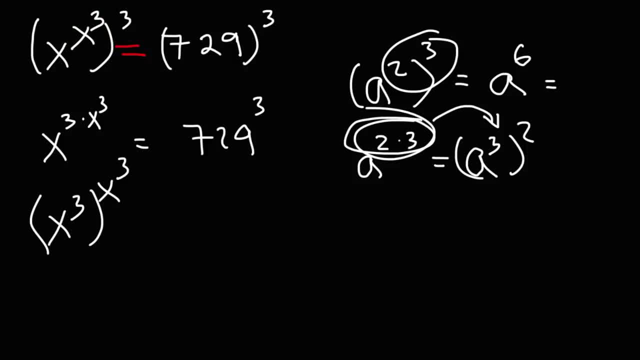 to the 2 and the 3.. And we can do that. Mathematically both expressions are still equivalent, But notice that these two are in the same form. They're equal to each other- x cubed raised to the x cubed- And so what we want to do now is change this expression such that we have: 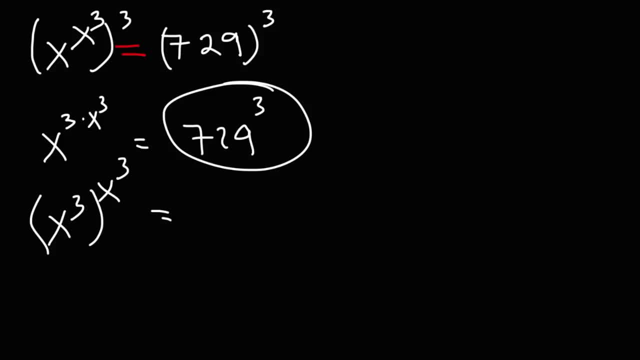 a number raised to the same number. If we can do that, it's going to make this problem a lot easier to solve. 729 is a cube of what number? 9 times 9 times 9 is 729.. So it takes three 9s to multiply or to get. 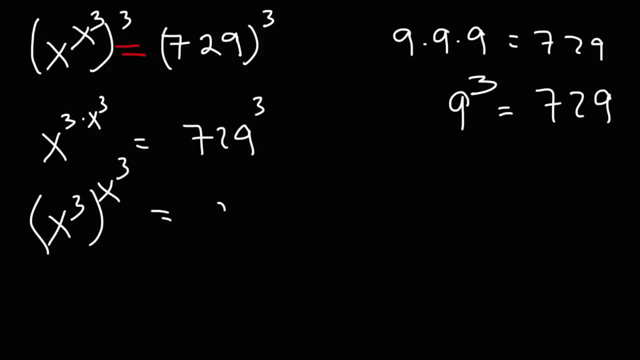 to 729.. So we can replace 729 with 9 to the 3rd power, And so we have this. Now, once again, we have an exponent raised to another exponent, So we can multiply those two numbers 9 times 3 is 9.. So we have x cubed raised to the x cubed, And that's equal to 9 raised to the 9th. 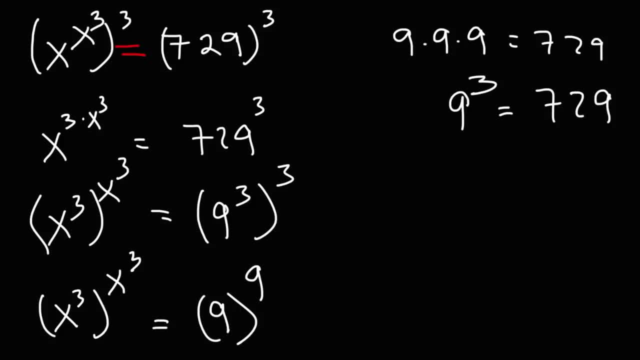 power. So now that we have a number raised to the same number, we can clearly see that that number is equal to x cubed. So x cubed is equal to 9.. Now, what is our next step here? What is the value of x? 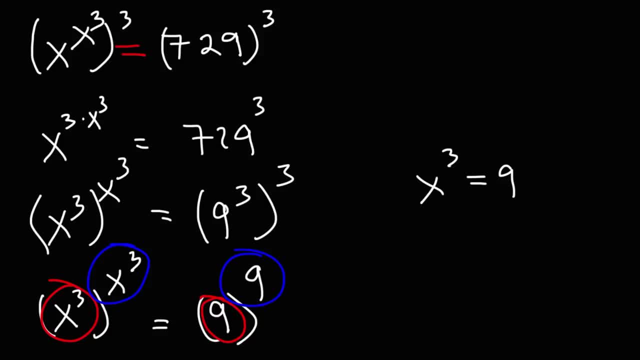 Given that x cubed is equal to 9.. To get x by itself, what we need to do is raise both sides to the 1- 3rd power 3 times 1, 3rd is just 1.. So we get x to the 1st power, which is simply x. 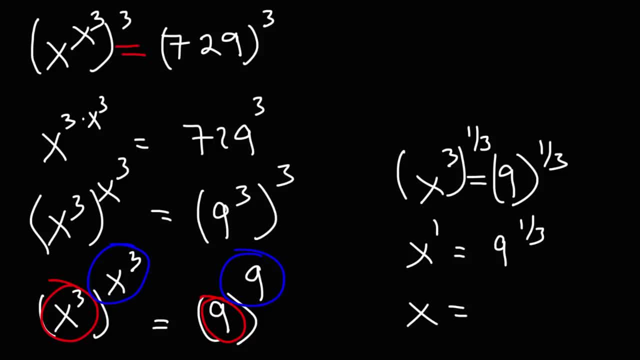 And 9 raised to the 1, 3rd, we can convert the fractional exponent into a radical. So this is the cube root of 9.. And so that is the answer. x is equal to the cube root of 9.. And you can check the work by plugging into the original expression. 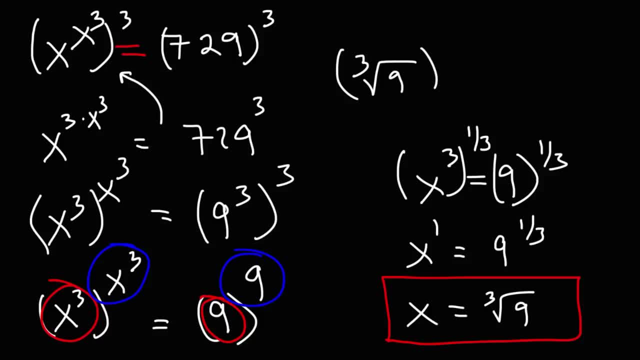 So the cube root of 9 raised to the cube root of 9, raised to the 3rd power, that should equal 729.. And you can plug that in your calculator to confirm that answer. So this is the final answer. Now you know how to solve this particular type of exponential equation. Thanks for watching. 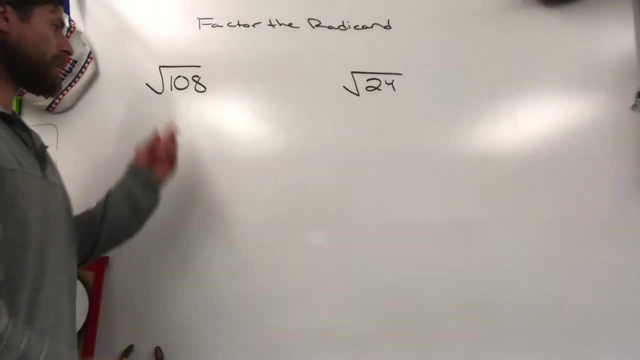 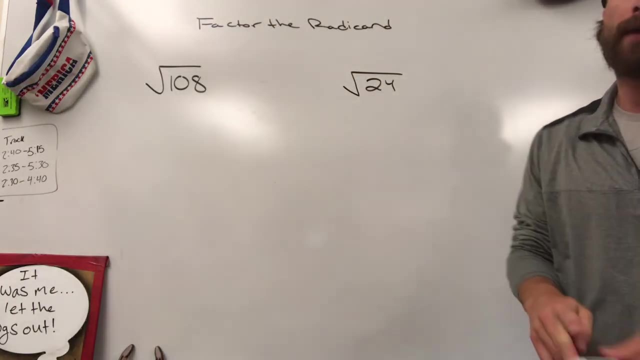 All right, let me teach you how to factor these. So we've got square root of 108, square root of 24, neither of which are perfect squares. So to simplify these down or to factor them out, all we got to do factoring right, Splitting something into two things. that, when 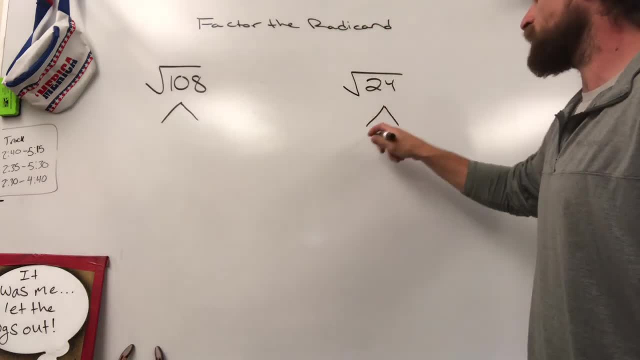 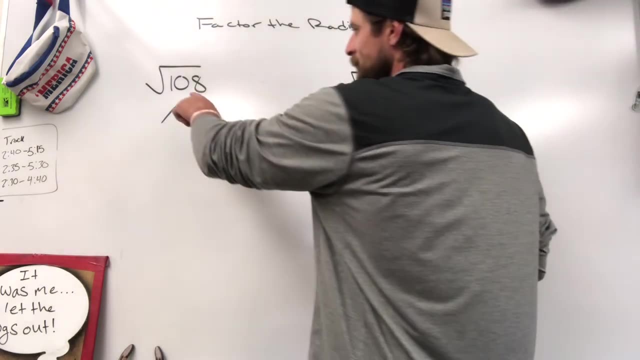 multiplied together would bring you right back to it. So that's what we're trying to do Now. if we're simplifying this, we need to make it neater, right? That's our whole job of simplifying Now. I could take 108 and divide it by two, right, But if I take it and divide it by two, 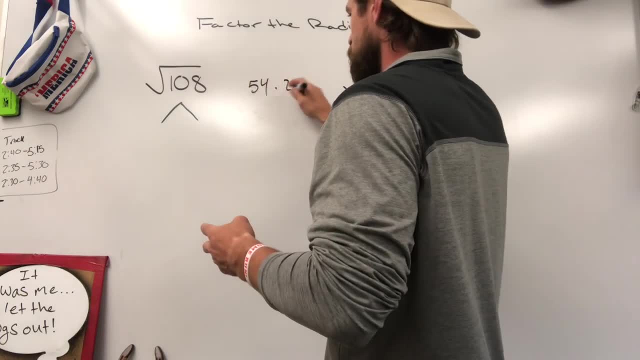 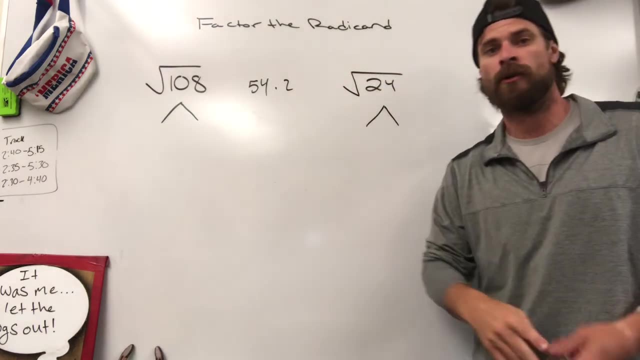 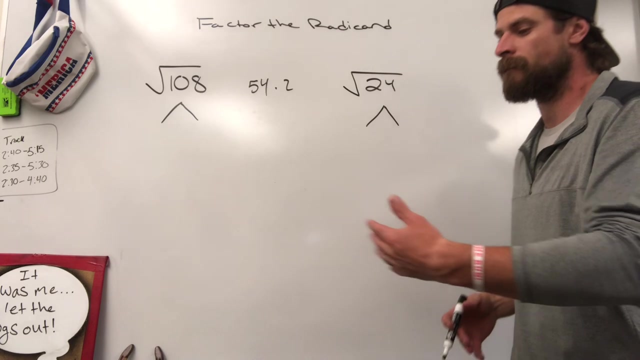 I'm going to get a 54 and a two, neither of which are perfect squares, okay, So we should know by now our perfect squares. We should have that list memorized, you know: 4,, 9,, 16,, 25,, 36,, 49,.